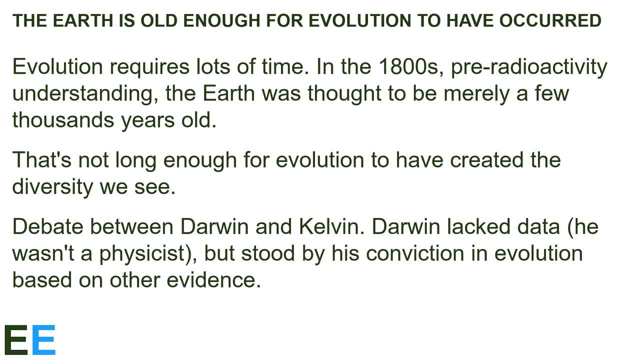 the data to demonstrate that physicists were incorrect, because he wasn't a physicist, but he stood by his conviction in evolution based on other evidence, including the fossil record. This disagreement about the age of the earth was a major problem for evolutionary theory in the 1800s. 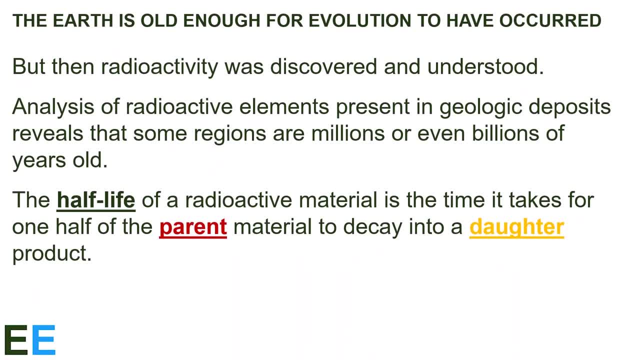 But then radioactivity was discovered and understood. The analysis of radioactive elements present in geologic deposits revealed that some regions were millions or even billions of years old. The arguments of biologists were vindicated and physicists had to adjust their view of how old the earth was. 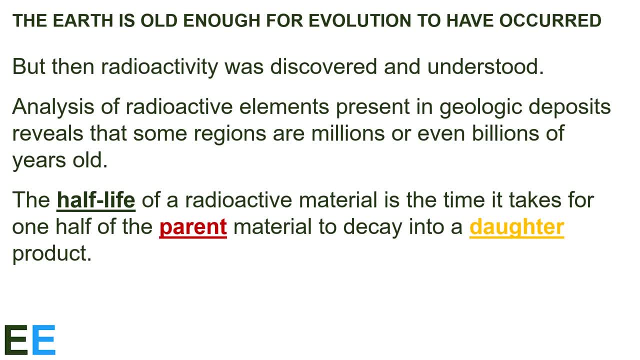 So how are radioactive materials used to estimate the ages of geologic deposits? Radioactive materials break down over time into less radioactive materials. The half-life of a radioactive material is the time it takes for one half of the parent material to decay into a daughter product. Each atom is on its own, with a certain chance. 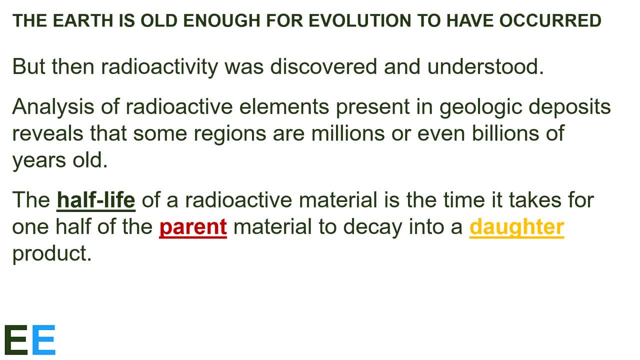 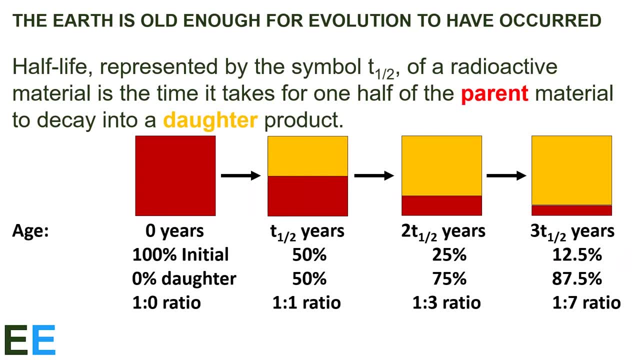 of decaying over time, and the half-life measures how long it takes for half of those atoms to do so. Let's look at radioactive decay in a little bit more detail. As mentioned, the half-life represented by the symbol T sub 1 half of a radioactive material is. 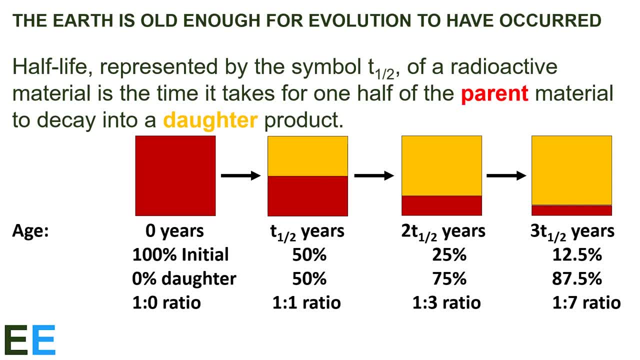 the time it takes for one half of the parent material to decay into a daughter product. Let's look at this diagram and think about what it's representing. The red box on the left indicates an initial amount of radioactive material. Let's give it an age of zero years when it begins to decay. At that initial point we 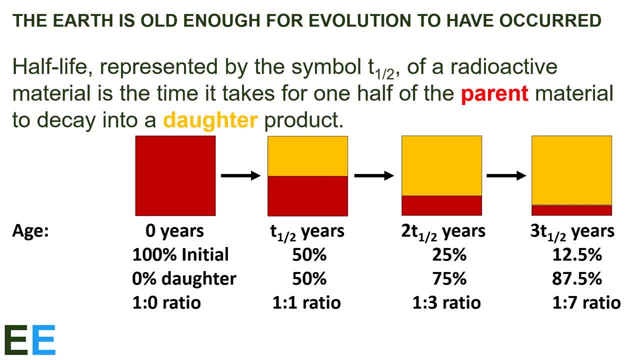 can think of 100% of the material being the initial element and 0% being the daughter element. We can also think of this as a 1 to 0 ratio. Ratios are often confusing to work with, but they're commonly used After one half-life, which 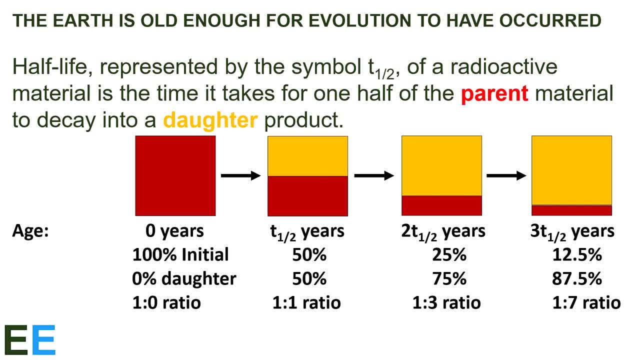 is T sub 1 half years, half of the parent material decays into the daughter product. If we look at our initial deposit now, 50% of the deposit is the initial material and 50% is the daughter material. That can be represented as a 1 to 1 ratio After an additional half-life. 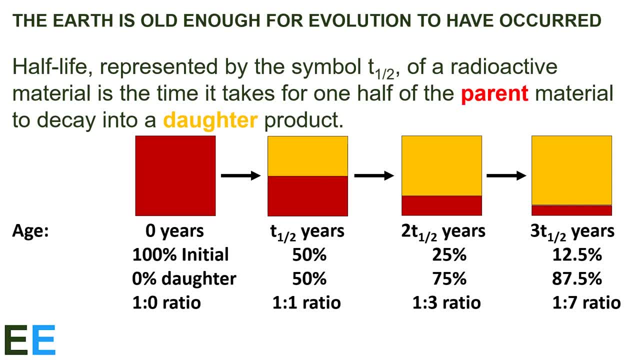 number of years, or twice the half-life number years from the beginning. there would now be just 25% of the initial material remaining. The 25 is half of 50.. Just because the atoms are older, they don't have a higher chance of decaying. 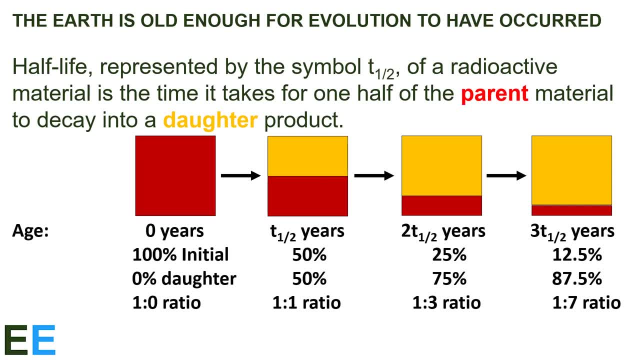 each year. Our deposit is 25% parent material and 75% daughter product. The ratio of materials would now be 1 to 3.. After an additional half-life number of years, or three times the half-life number of years from the: 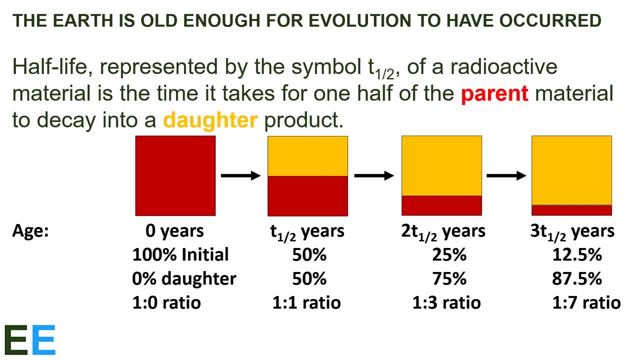 beginning now, there would be 12.5% of the original material remaining. The 12.5 is half of 25.. Our deposit is 12.5% parent material and 87.5% daughter product. The ratio of materials would now be 1 to 7.. If we are 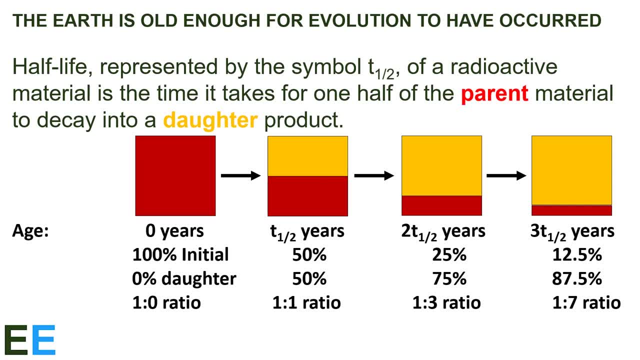 able to discover a deposit of radioactive material that has remained isolated from contamination, then a measurement of the relative amounts of the parent and daughter material will be계ission. to use this mapping, Naturaleчö gem, michère bentanum. if a lot of the materials are still alive, TheSe blindness matrix will be the domestic. another characterization that can be examined in active Mo資 mission operation. 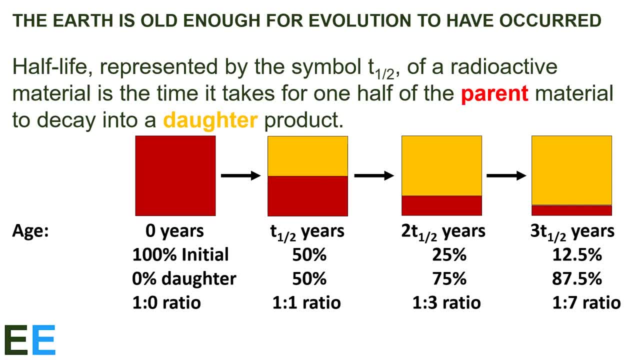 Then a蹤 t специ exposedEEP. Specialization in Im mantle and logique interpretation ofkten development will tell us how long ago that initial deposit was formed. Finding such deposits and carefully measuring these ratios is something that geologists do to estimate the ages of different layers of rock. 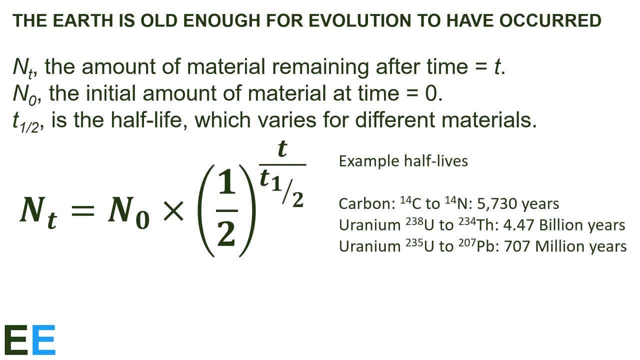 Of course, in reality, the ages of these deposits are rarely nice multiples of the half-life, so we have to use an equation like this to estimate the age of a deposit. This equation shows that the amount of the material after a certain amount of time. 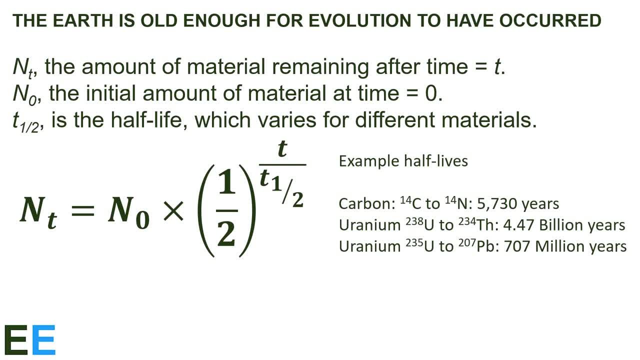 is equal to the initial amount of the material times one-half raised to a power, which is the amount of time divided by the half-life. For example, once the time equals the half-life, that exponent is one and the amount of material would just be equal to the initial material times one-half. 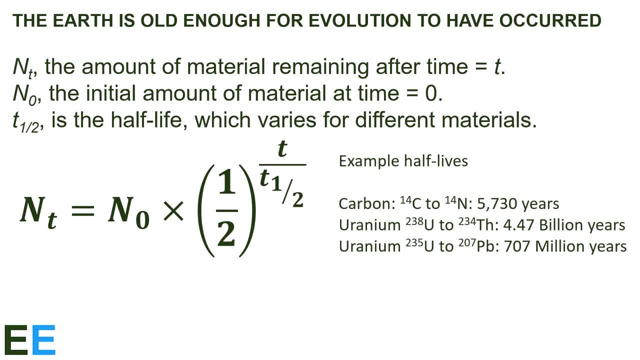 If the amount of time was twice the half-life, the exponent would be two and the amount of material would be equal to the initial amount times one-half squared, which is one-fourth. Using this equation becomes very difficult in practice if the time is a large multiple of the half-life. 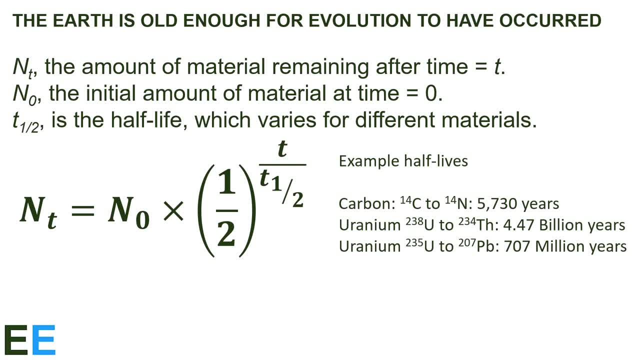 because the time is very small, Because the amount of measurable material is too small. Luckily, there are a variety of radioactive materials that have a range of half-lives that allow us to accurately date many different deposits. For example, the decay from carbon-14 to nitrogen-14 is about 5,700 years. 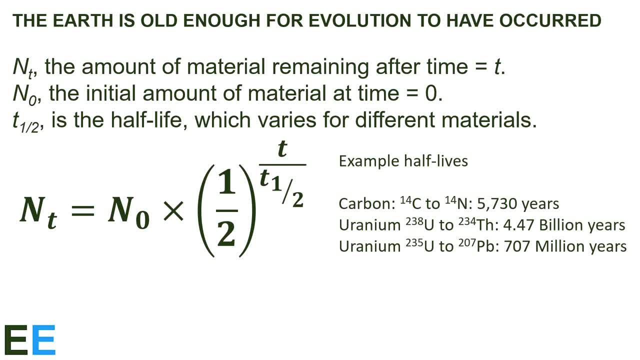 so deposits of carbon that start with a known amount of carbon-14 can be used to accurately date things up to about 30,000 or 40,000 years old. This is perfect for learning about early humans who left carbon deposits in their ancient campfires. 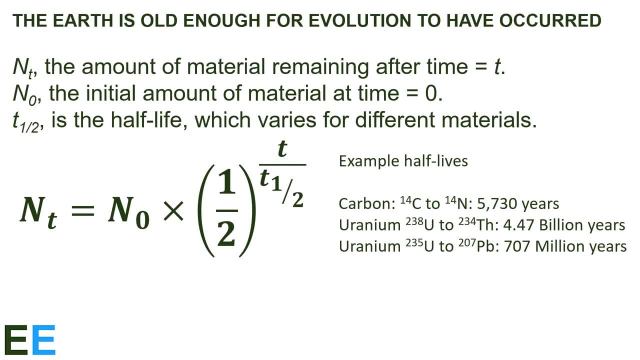 At the other end of the scale are isotopes like uranium-238 and uranium-235 with half-lives that are millions of years old, which allows us to date very ancient deposits, And once physicists and geologists figured all this out and started measuring isotopes of uranium, thorium and lead in rock formations. 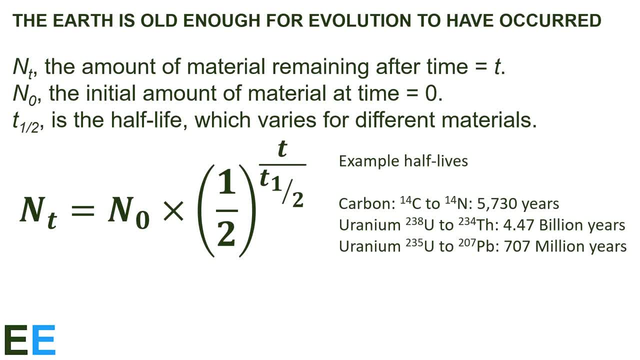 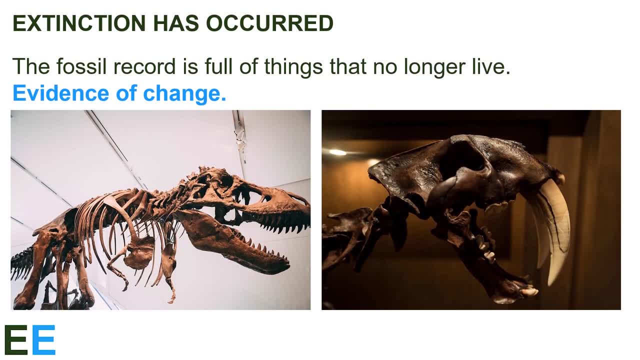 they came up with ages that were ancient. This then indicated that the Earth was plenty old enough for evolution to have had time to occur. In addition to providing estimates of the age of rocks, the rocks themselves show us things that lived before via fossils. 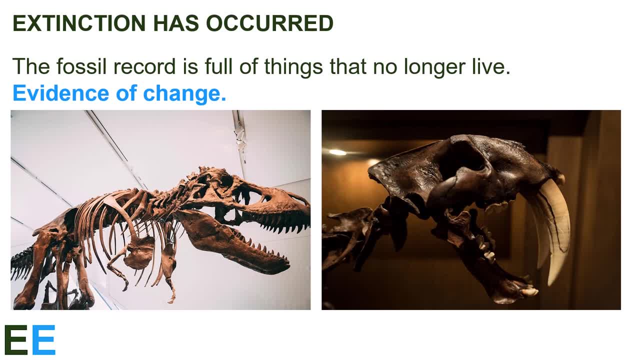 the preserved imprints of things buried long ago, And one of the most obvious things is that the fossil record is full of organisms that no longer live. Extinction has occurred during Earth's history- Animals like the Tyrannosaurus rex and saber-toothed cat shown here. 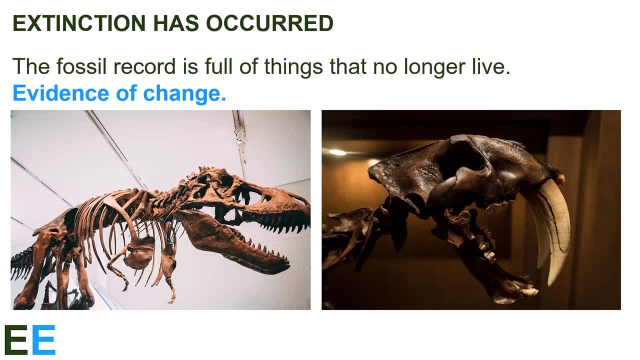 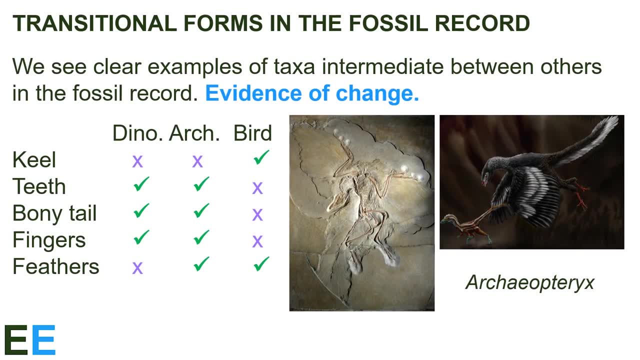 are very different from things alive today. This is evidence of change. The organisms on Earth have not always stayed the same. We also see clear examples of tacks at intermediate between others in the fossil record- more evidence of change. For example, the fossil shown is Archaeopteryx. 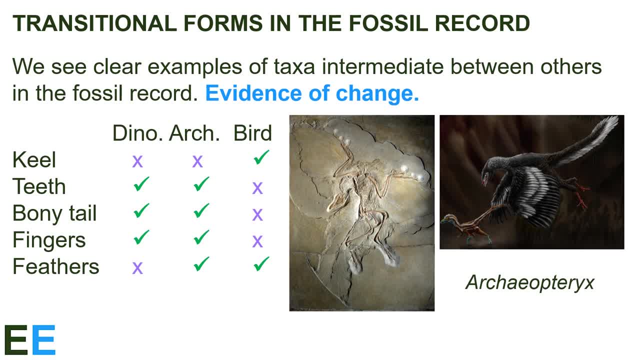 and you can see the artist's rendition beside the fossil. This is such an important fossil because it shows us what a transition looked like. Dinosaurs, which are reptiles and birds, are very different from each other. Dinosaurs do not have a keel. 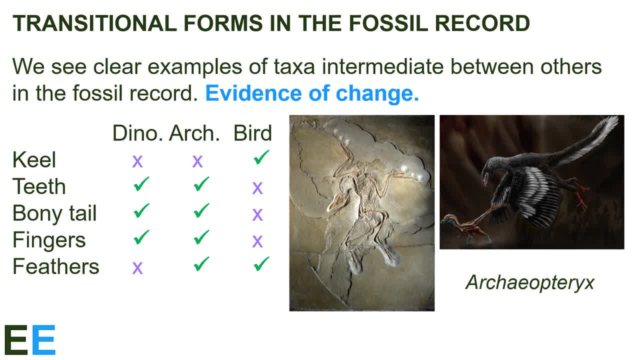 the large extension on the breastbone that wing muscles attach to. nor do they have feathers, But they do have teeth, a bony tail and separate fingers in their forelegs. Birds do have a keel and feathers, but birds don't have teeth or bones in their tails. 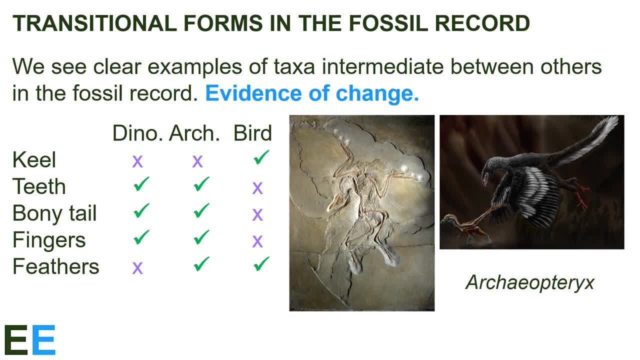 and the fingers in their forelegs are fused together into little nubs. Archaeopteryx exhibits a mix of traits that show the transition between these two organisms. The fossil of Archaeopteryx shows that it does have feathers like a bird, but the rest of its features are different from a bird and more like a reptilian dinosaur. 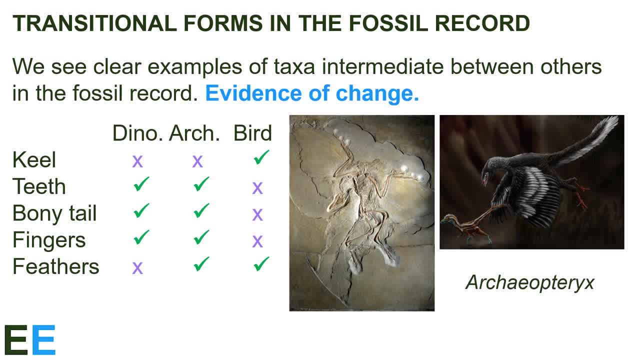 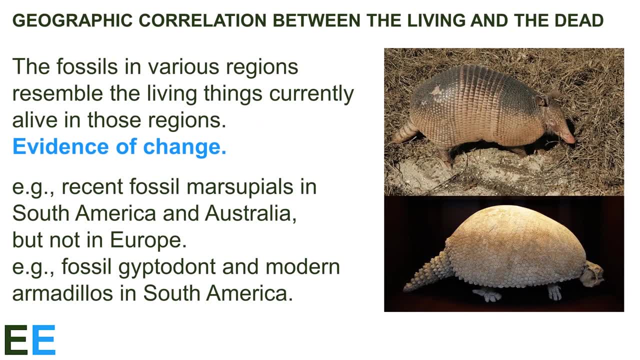 This fossil shows an organism that is clearly in transition between a previous organism and a subsequent one. And finally, the fossils in various regions resemble the living things currently alive in those regions. There is a connection and relationship between today's living things and what used to live in the same location.